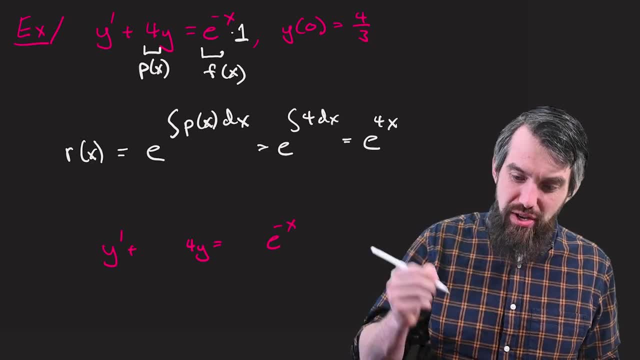 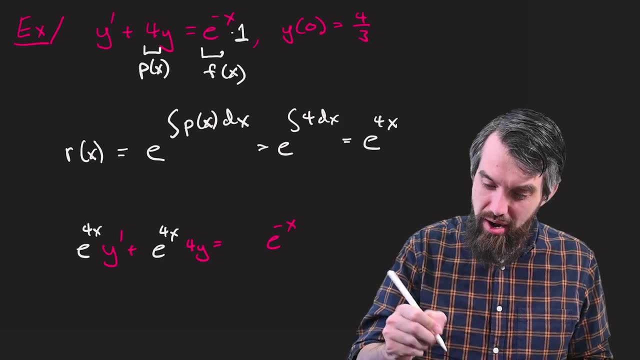 of a space there and a little bit of a space there, and the method is going to be the same. The method of integrating factors is all about taking every single term and multiplying by that integrating factor. I'll put an integrating factor there, there and there. Maybe I'll just 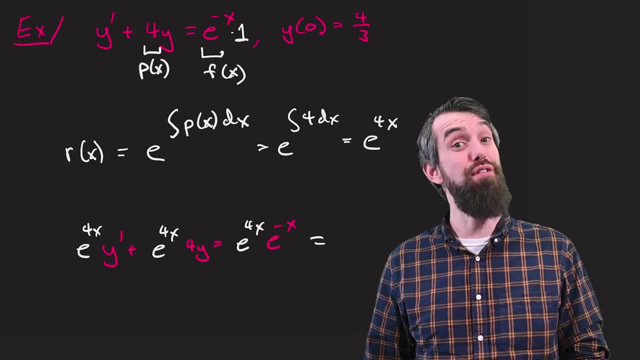 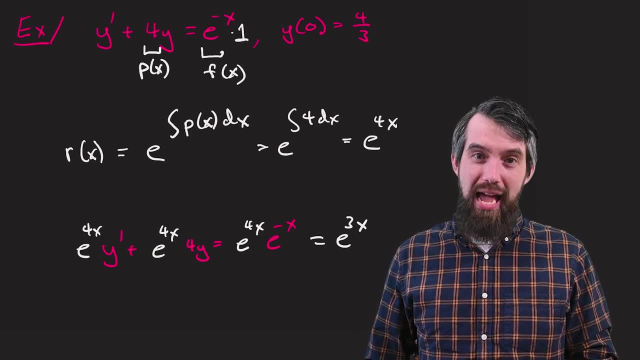 do a little simplification on the far right hand side and see that e to the 4x times e to the minus x is the same thing as e to the 3x. I can simplify that on the right hand side. Now the next step is: 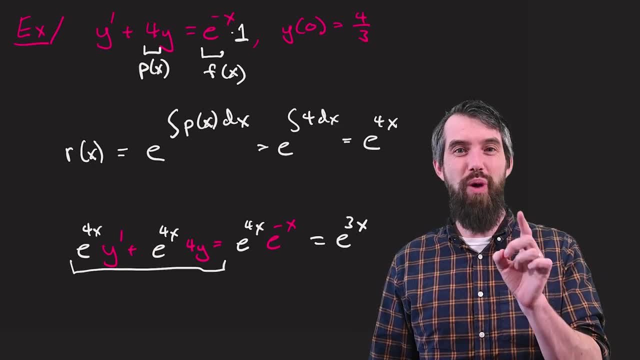 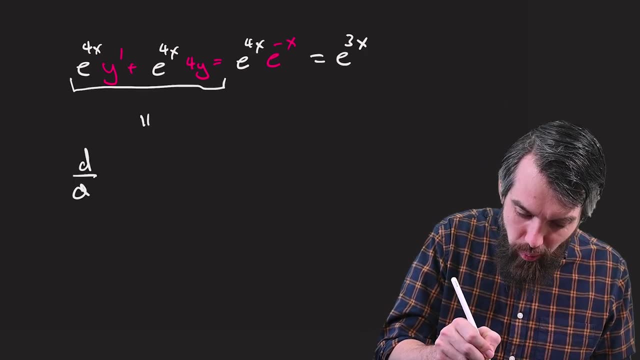 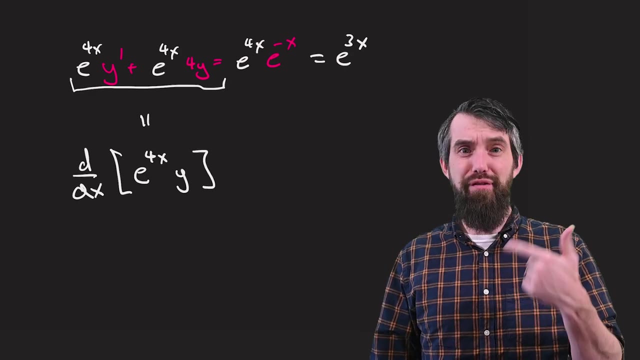 to simplify the left hand side- and this is where it gets kind of interesting- I'll notice that the this is the same thing as the derivative with respect to x, of e, to the 4x multiplied by y, and you can verify by the product rule that you'd get exactly that. and indeed when we introduced 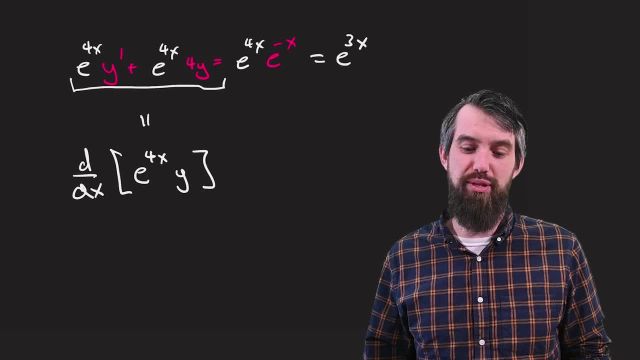 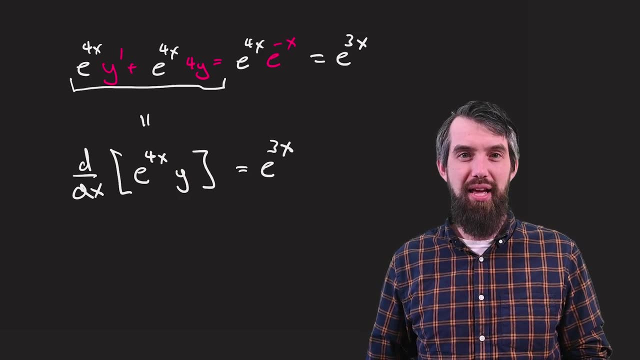 this method of integrating factors. we defined the integrating factor, so this would always be true, so it was always going to be the case. it was the derivative on the left hand side, and then some function which is on the right hand side. Okay, so now I'm going to integrate. 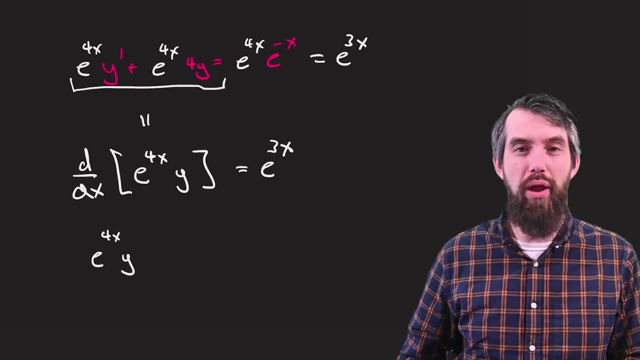 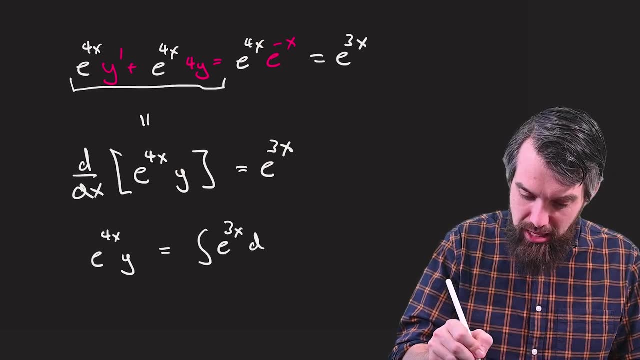 and that's going to give me, on the left, e to the 4x times y. all I'm doing here is just integrating a derivative so it cancels. and then this is the same thing as the integral of e to the 3x dx, which is 1, 3rd times e to the 3x. and now I am going to write: 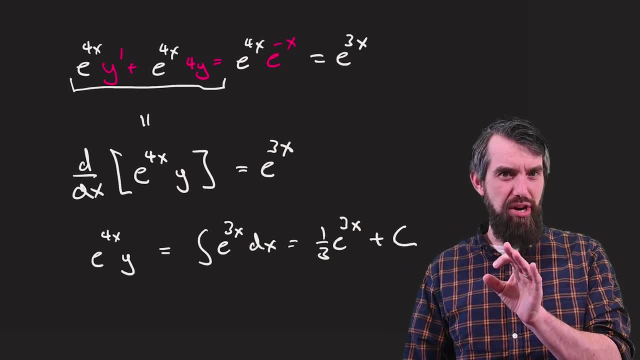 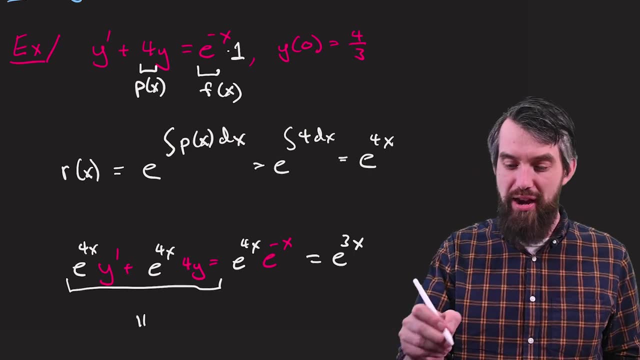 down a plus c. You might think this is a little bit odd. I told you earlier you didn't need to write down the plus c, but you didn't need to write down the plus c earlier because it was all about finding an integrating factor, and in an integrating factor we just wanted any one. that 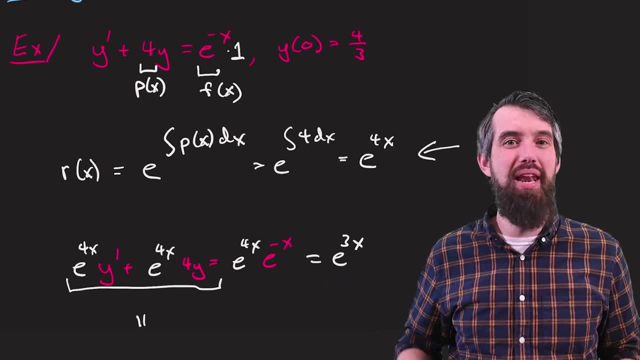 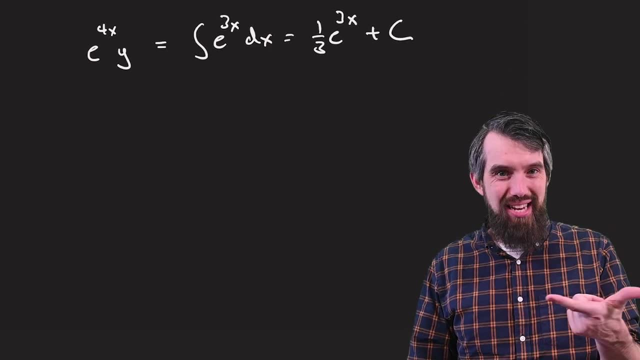 worked. Indeed, if you had a plus c that was sticking out there, it would have canceled the next line anyways. But now I'm going to my solution, and what I've gotten is this expression that has an indefinite interval. I do want my plus c, and my plus c will be useful for 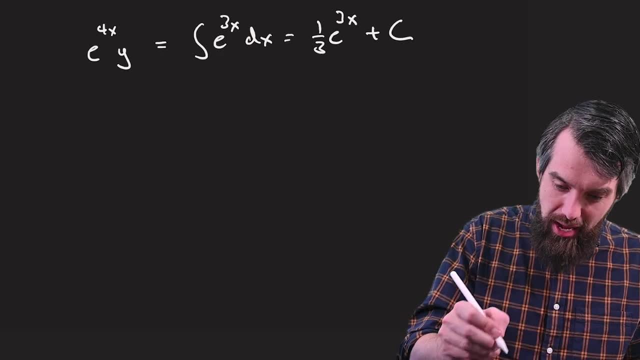 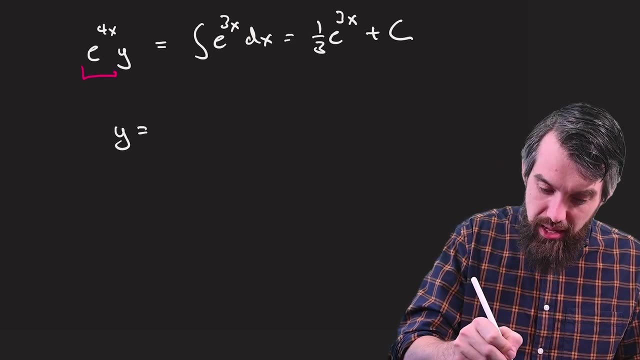 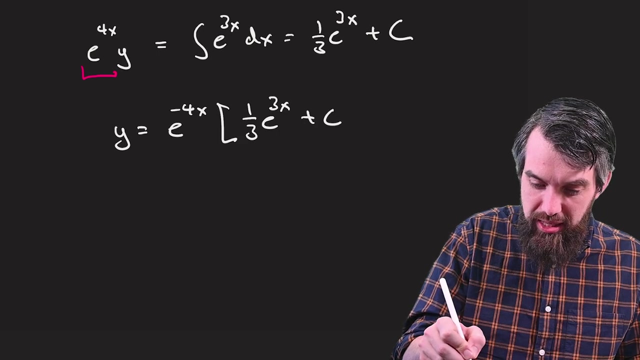 my initial condition. Well, final answer. I noticed that I have this e to the 4x stuck still on the left hand side. I don't want that, and so I'll say that y is going to be e to the minus 4x multiplied by the 1, 3rd, e to the 3x plus the c. and if you prefer to distribute this,